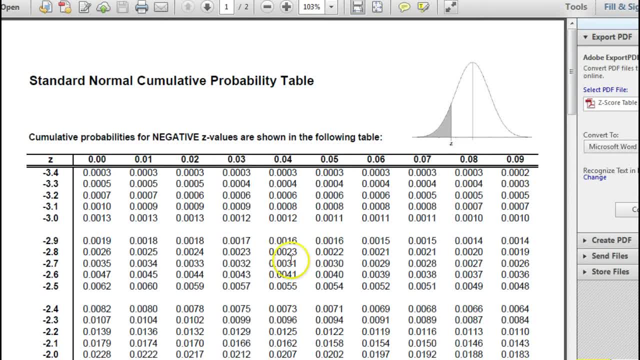 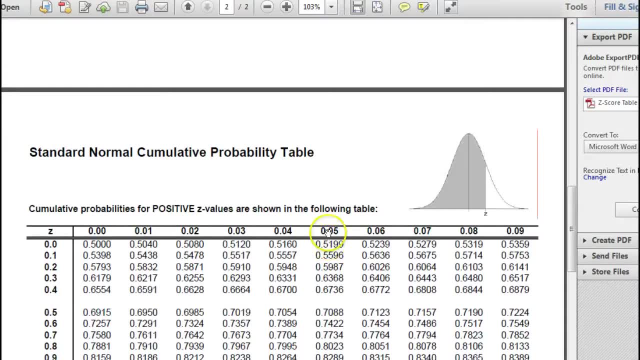 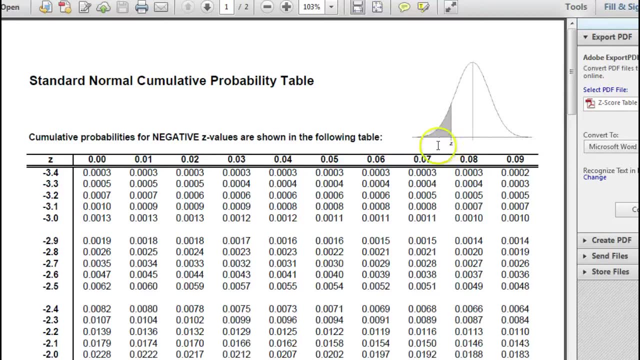 going to use this chart of z-scores, So if you don't have one of these z-score tables, then you need to google it and download one, because you need this to be able to answer these types of questions. Okay, now, this is a chart of z-scores, So we're going to need the z-score instead of 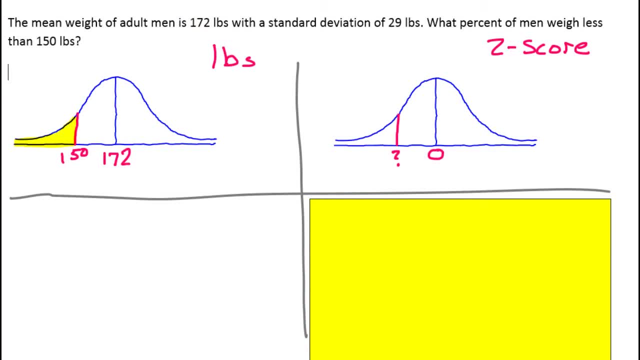 pounds. So the way you convert over- and I'm temporarily going to borrow this area for the formula- It's not really what goes over here, but the formula for z-score is like this: You take any value, you subtract the mean and you divide by the standard deviation. 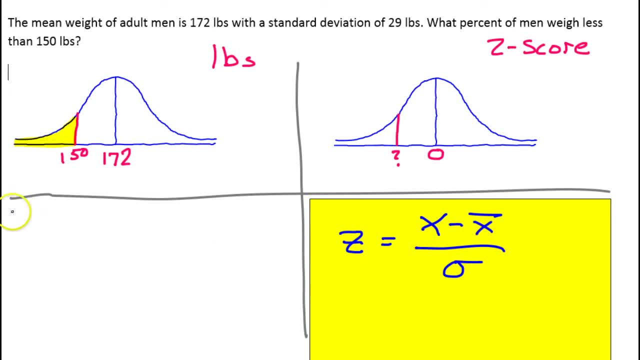 So that's the formula. So let's do that right now. So to find the z-score, I'm going to take my value of 150, I'm going to subtract the mean and I'm going to divide by the standard deviation. 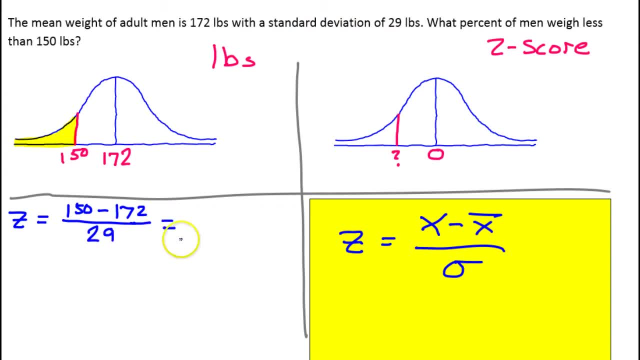 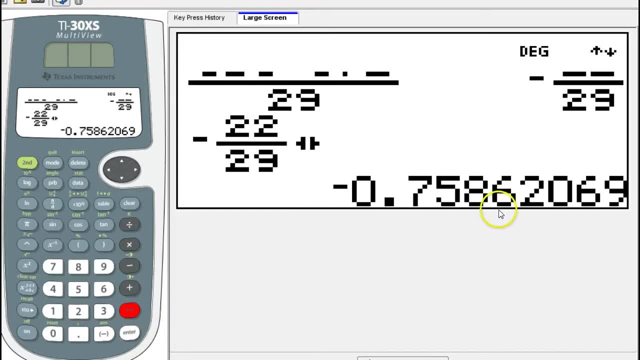 which was 29.. And let's see what we get. Okay, so here we go Now. for z-scores, we're always going to use two decimal places, So we're going to have to kind of cut it here. Now, rounding is going to be very important, Because this next number is 5 or greater. that means this: 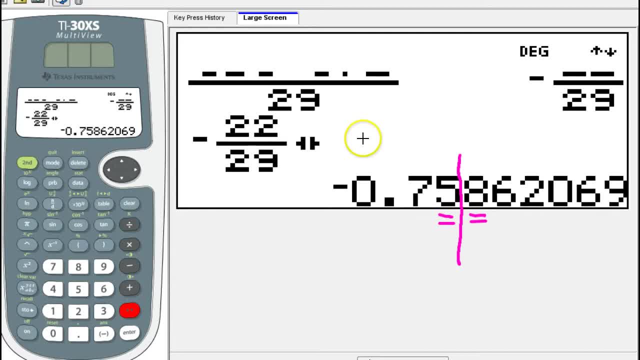 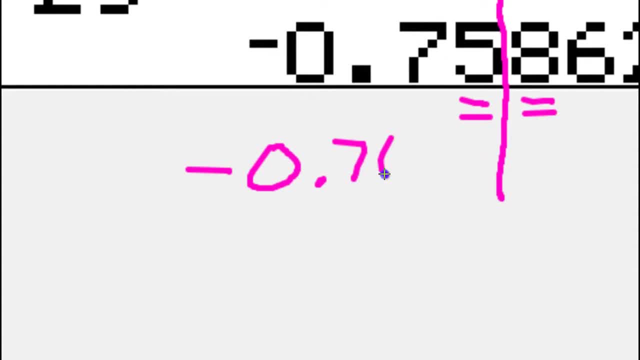 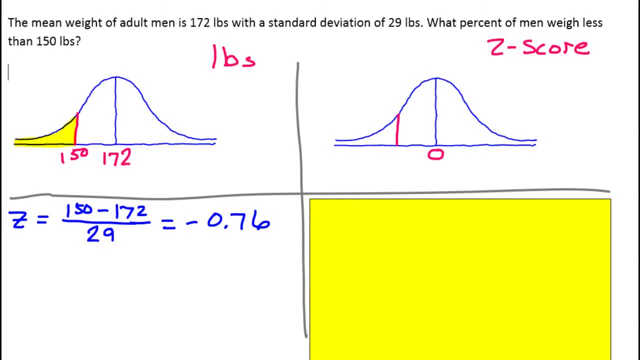 number is going to have to be rounded up, So our final answer should be negative 0.7,. oh, negative 0.76.. because we have to round up, Okay, so we have our z-score of negative 0.76, and just like on our pounds diagram, 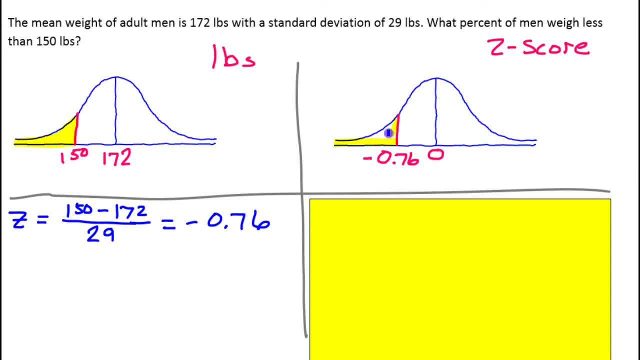 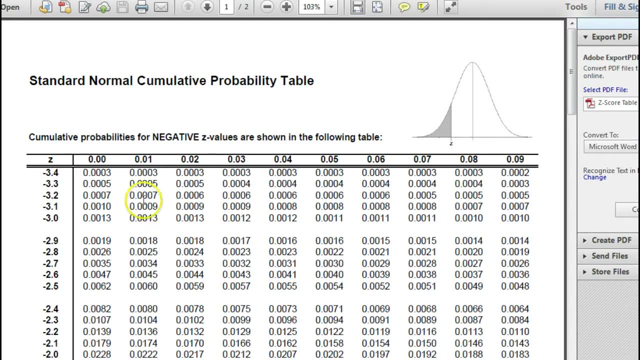 we want to find the percentage of z-scores to the left of this one, And here's where the chart comes in. This shading here reminds us that this table of values gives us the percentage of z-scores to the left of 1.. 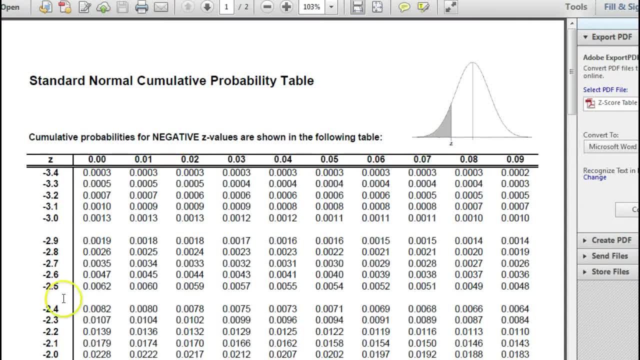 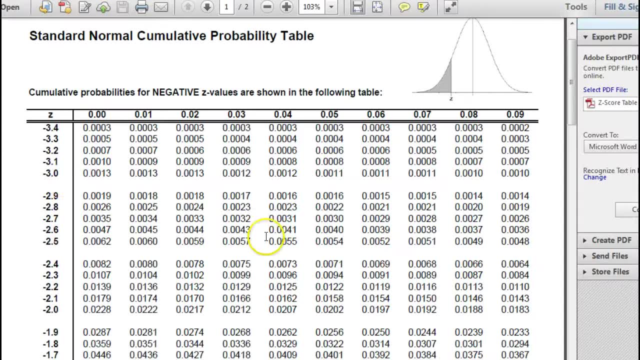 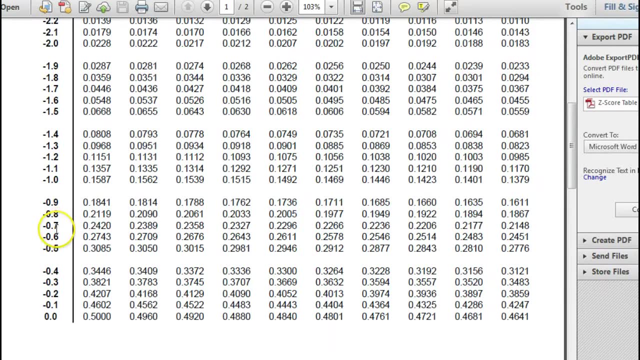 of any particular z-score. So all we have to do is find the z-score that we are interested in over here on the left. So we want negative 0.76.. Okay, so let's see, negative 0.7 is right here.